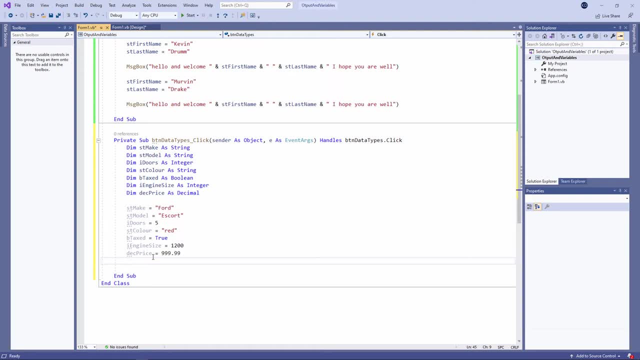 to store money values. I could have used double and I could have used single, because all three data types- decimal, double, single- allow me to have a decimal point with decimal places after it. But double is twice as accurate as single Because double is twice as easy to get for. 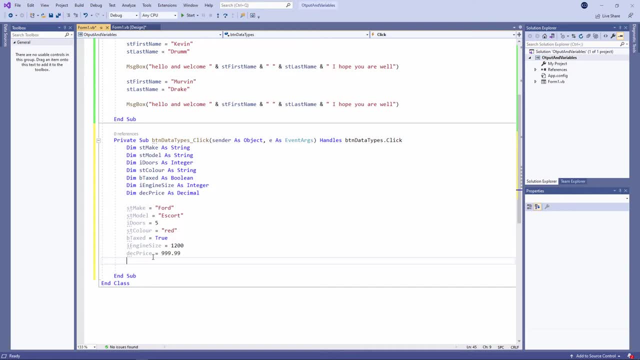 less vegetables. my data type is a centre and just size is wirklich needed to build my property. So in order to store all the data types, I would need to be able to store single. I can have more decimal places and the data type decimal is the most. 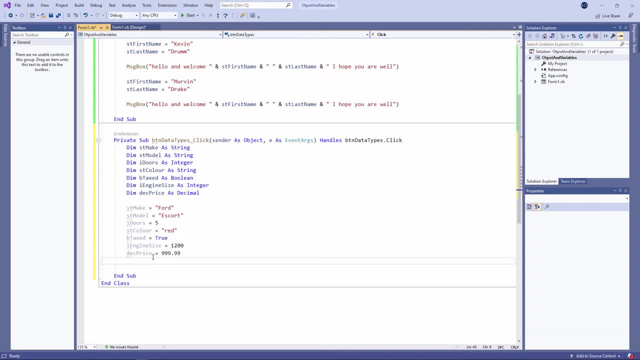 accurate of them all, which makes sense when you're doing calculations with money. the final thing I want to store is the date that the car was registered, so I'm going to use a data type of date. there's a special way that I have to assign a value to a date variable. notice. 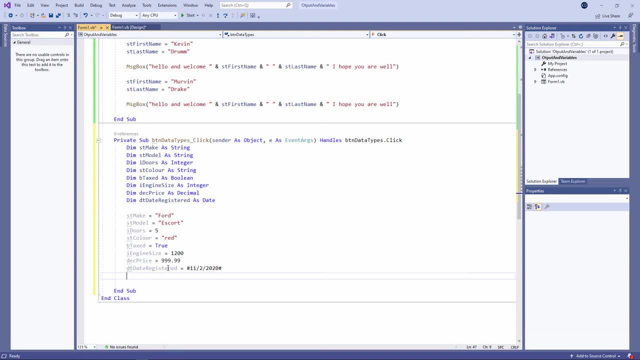 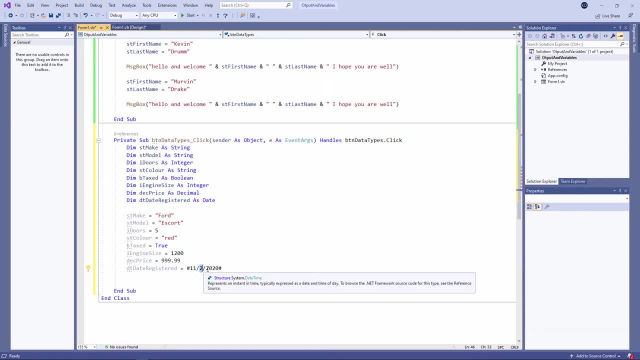 followed by the day, followed by the year. when I display this on the screen, for example in a message box, it'll be displayed according to the settings in my computer's control panel. you'll see in a moment that my computer is set up to display dates in British format. now let's build a message box command to: 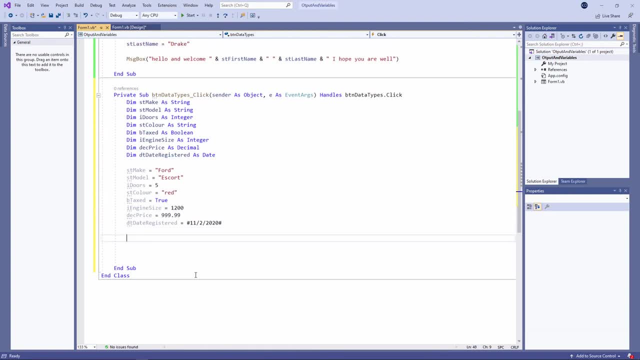 display all of this data. you notice the concatenation operators between the variable names and notice also that I'm concatenating spaces between these data items. now you can see I have a bit of a problem here with reading the code I've written on the screen. nevertheless, let's test it and see if it runs. there's my message and it looks. 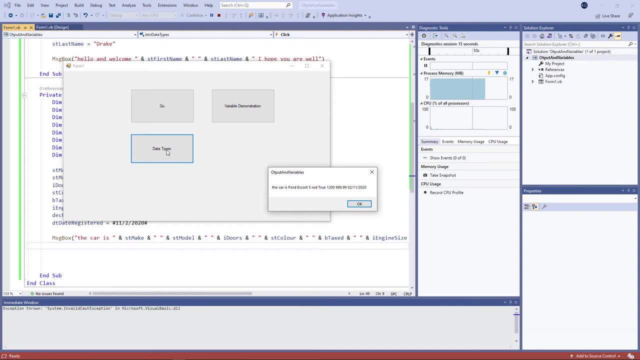 okay, notice that the day and the month of the date are the other way round from the way I coded it. I've written the date in American format, but it's being displayed in British format. what I'd really like to be able to do is display each data item on a separate line within the data item box, so that I can display each data item on a separate line within the data item box. 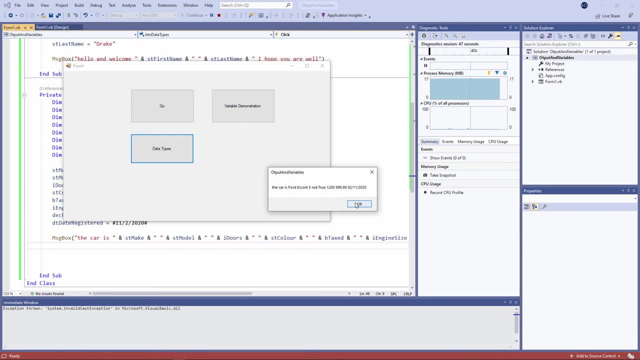 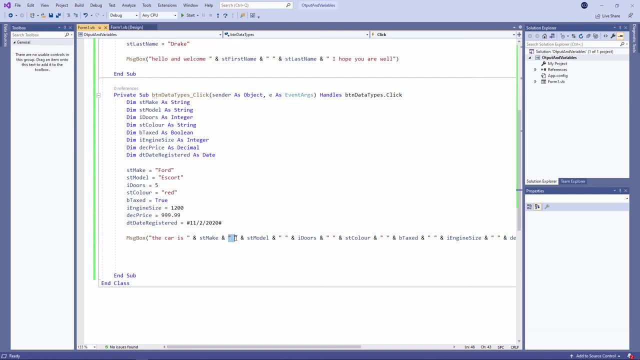 the same message box. let's see how to do that. instead of concatenating spaces in between each data item, I'm going to type a special constant. I'll say more about constants later. suffice to say: I'm just going to type VB, new line, and I'll replace each space with this. let's just copy and paste it. ctrl C to copy ctrl block. here I'm taking a wash� call. I don't know if it's just screen not lying on the screen. will it just say and look, nevermind if that's what we're doing, its just ruined the message. it said: beat наши sjew dunno das hier 뭐야 decachat. 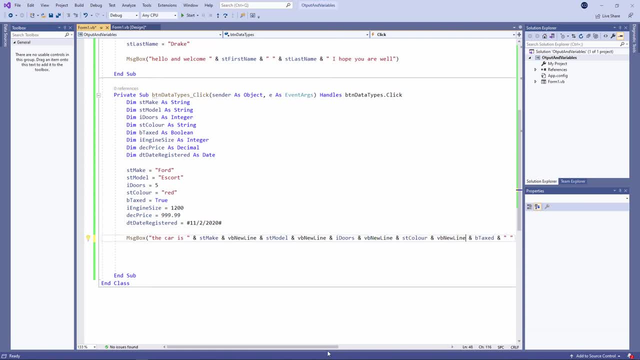 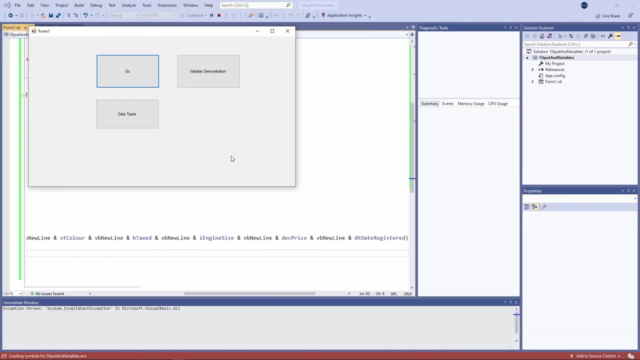 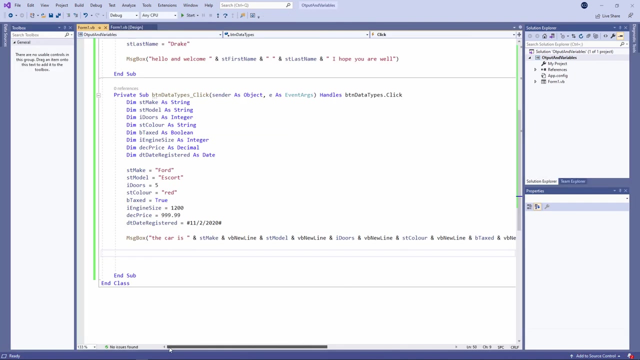 I still need the same number of concatenation operators to join all these different bits and pieces together. Let's see how it looks now. Well, that is certainly a nicer message, But now I want to do something about the problem that I can't actually read the whole line. 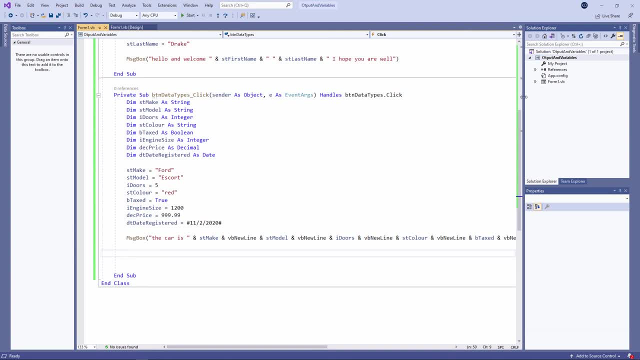 of code. I could give myself some more space on the screen by just dragging this bar across a little bit, but even then I can't read the whole line of code. I essentially want to wrap this text on the screen. Well, I can do this. 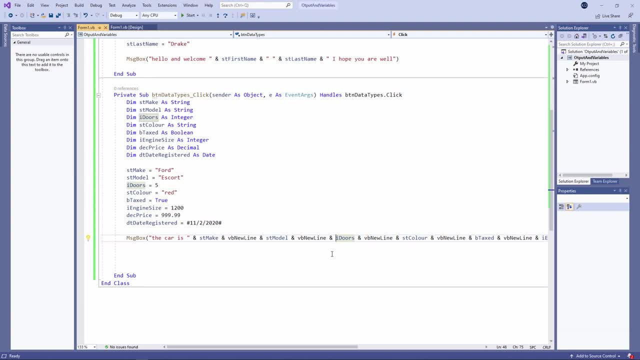 After the ampersand. here. in fact, I can put this pretty much anywhere. I'm just going to leave a space and then type an underscore character. When I press enter, I've moved the rest of the line onto the next line. I can do that again here. 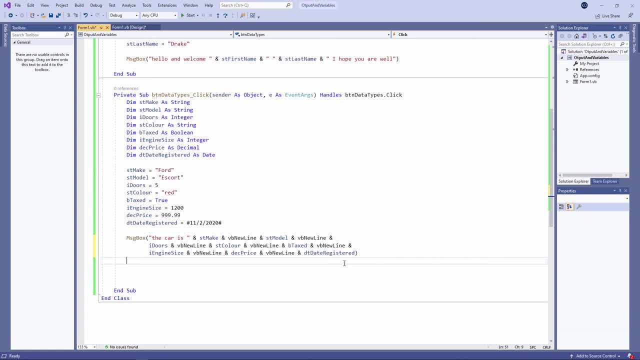 Notice the underscore characters have actually disappeared, but this is still just one line of code. It won't change the appearance of the message box, but it just allows me to read the code more easily on the screen. Let's make sure it still works.